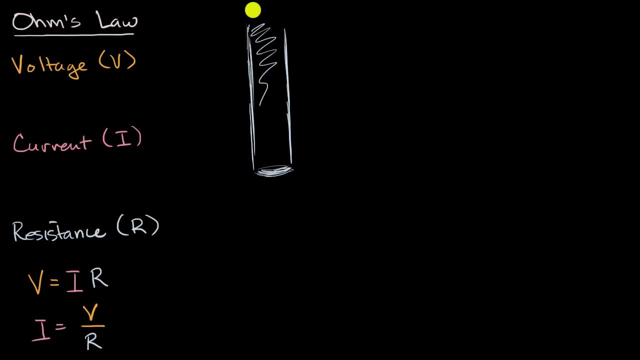 It's closed at the bottom right now and it's all full of water. There's water above here as well, So the water in the pipe, so let's say, the water right over here, it's going to have some potential energy. 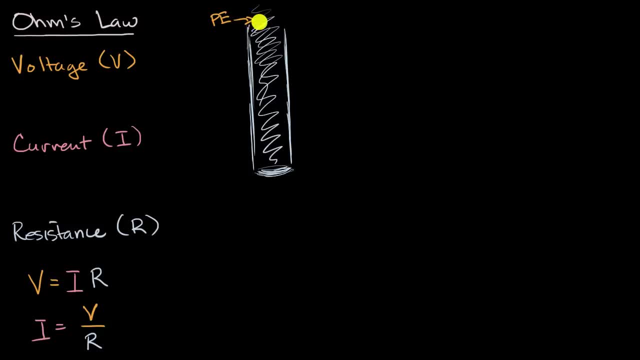 And this potential energy, as we will see it, is analogous. analogous to voltage. Voltage is electric potential, Electric potential. Now, it isn't straight up potential energy, It's actually potential energy per unit charge. So let me write that. 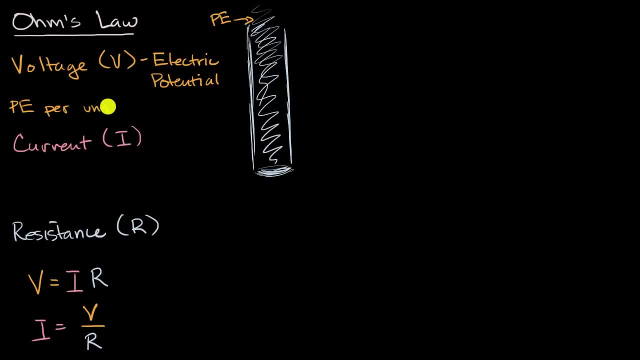 Potential energy per unit, unit charge. You could think of it as joules, which is potential energy, or units of energy per coulomb. That is our unit charge, And the units for voltage- for voltage in general- is volts. 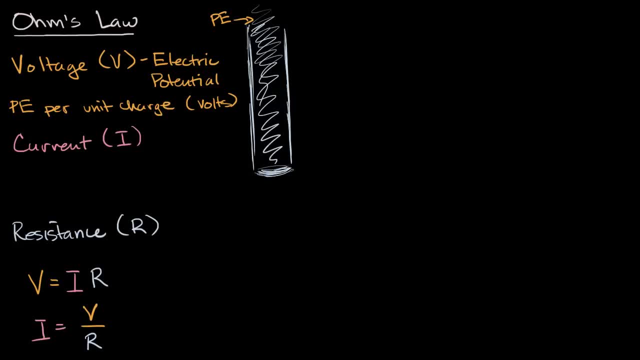 Now let's think about what would happen if we now open the bottom of this pipe. So we open this up. What's going to happen? Well, the water is immediately just going to drop straight down. That potential energy is going to be converted. 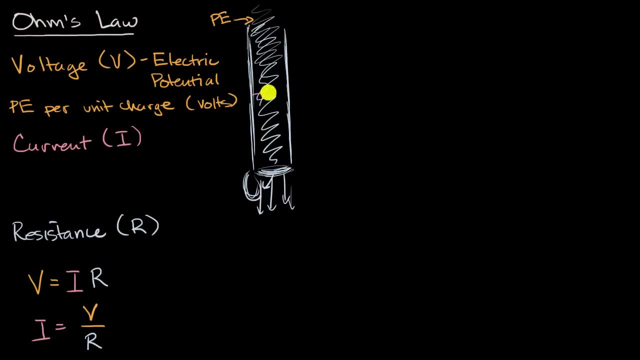 to kinetic energy And you could look at a certain part of the pipe right over here, right over here, and you could say, well, how much water is flowing per unit time And that amount of water that is flowing through the pipe at that point. 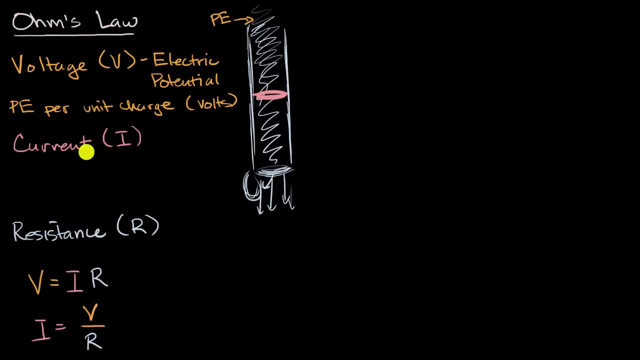 in a specific amount of time that is analogous to current. Current is the amount of charge. So we could say charge per unit time, Q for charge and T for time And intuitively you could say how much, how much charge flowing. 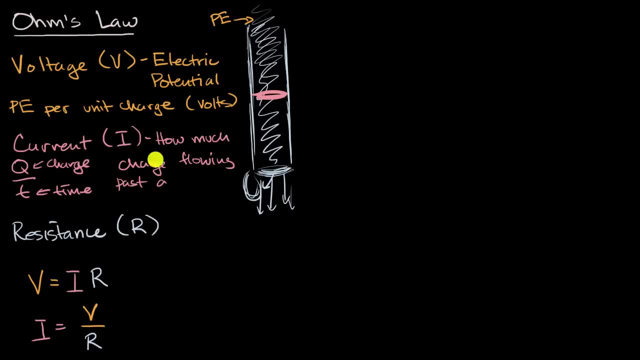 flowing past a point in a circuit, a point in circuit in a, let's say, a unit of time. We could use to think of it as a second, And so you could also think about it as coulombs per second: charge per unit time. 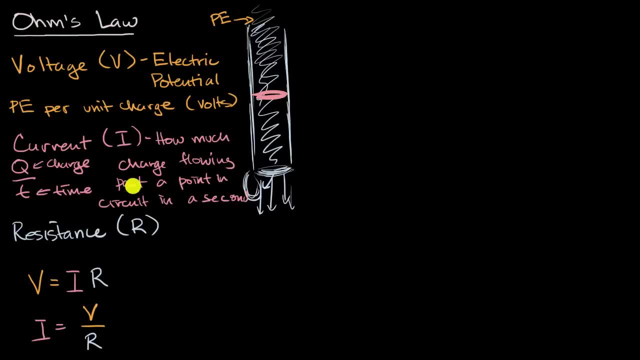 And the idea of resistance is something could just keep that charge from flowing at an arbitrarily high rate. And if we want to go back to our water metaphor, what we could do is we could introduce something that would impede the water And that could be a narrowing of the pipe. 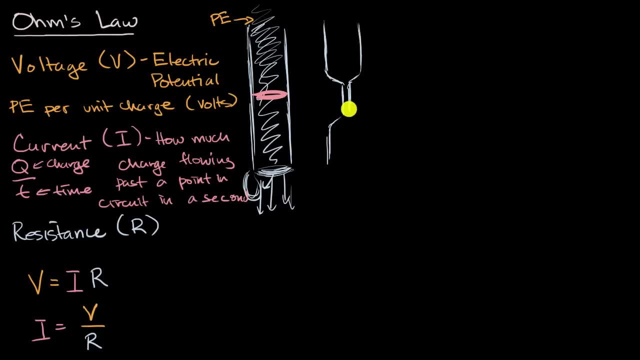 And that narrowing of the pipe would be analogous to resistance. So in this situation, once again, I have my vertical water pipe, I've opened it up And you still would have that potential energy, which is analogous to voltage, And it would be converted to kinetic energy. 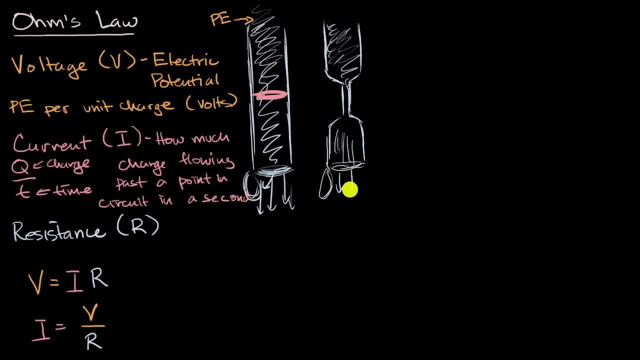 and you would have a flow of water through that pipe. But now, at every point in this pipe, the amount of water that's flowing past at a given moment of time is going to be lower, because you have literally this bottleneck right over here. 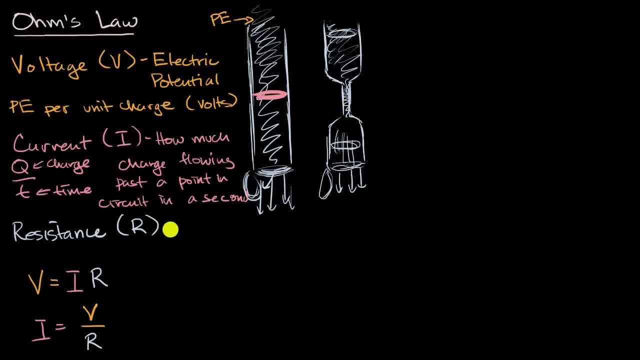 So this narrowing is analogous to resistance. How much charge flow impeded? Impeded, And the unit here is the ohm, Is the ohm which is denoted with the Greek letter omega. So, now that we've defined these things and we have our metaphor, 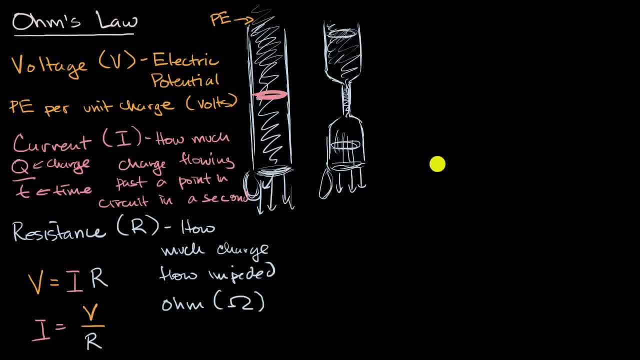 let's actually look at an electric circuit. So first let me construct a battery. So this is my battery And the convention is my negative terminal is the shorter line here, So I can say: that's the negative terminal, That is the positive terminal. 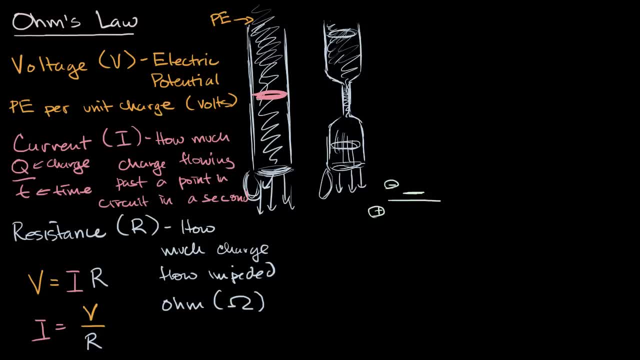 Associated with that battery. I could have some voltage And just to make this tangible, let's say the voltage is equal to 16 volts across this battery, And so one way to think about it is the potential energy per unit charge. let's say we have electrons here at the negative terminal. 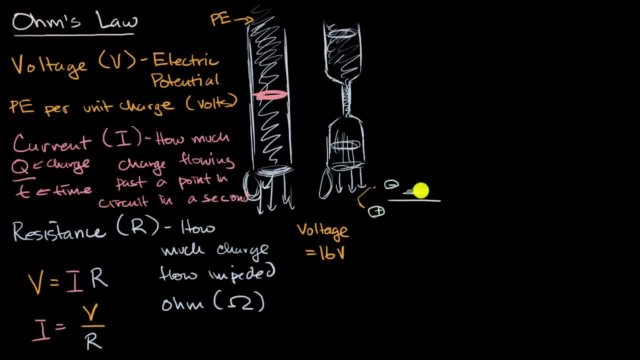 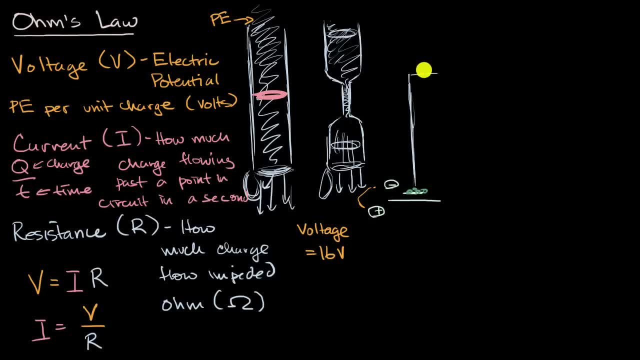 And so we can provide a path. So let me draw it like this: And at first I'm gonna not make the path available to the electrons, I'm gonna have an open circuit here, But I'm gonna make this path for the electrons. 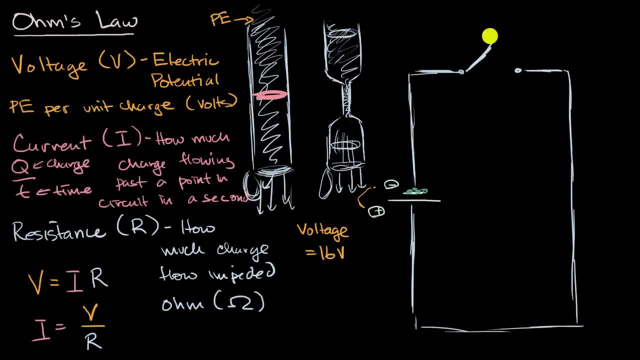 And so as long as our circuit is open like this- this is actually analogous to the closed pipe- The electrons- there's no way for them to get to the positive terminal. But if we were to close the circuit right over here, if we were to close it, then all of a sudden, 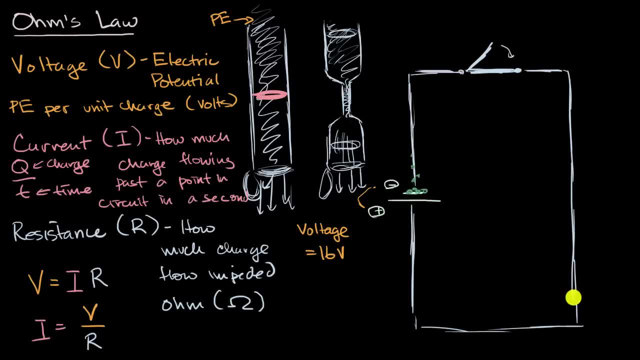 the electrons would go to the positive terminal. the electrons would go to the positive terminal, And so the electrons could begin to flow through this circuit in an analogous way to the way that the water would flow down this pipe. Now, when you see a schematic diagram like this, 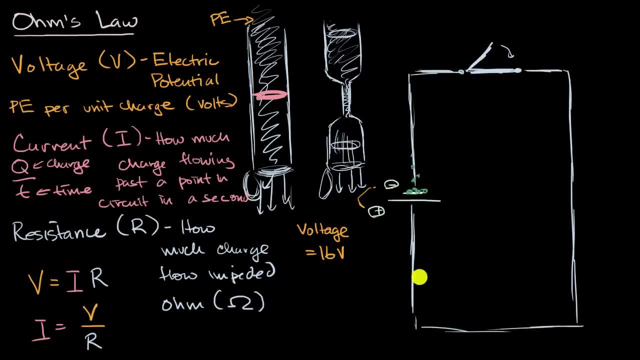 when you just see these lines, those usually denote something that has no resistance. But that's very theoretical. In practice, even a very simple wire that's a good conductor would have some resistance, And the way that we denote resistance is with a jagged line. 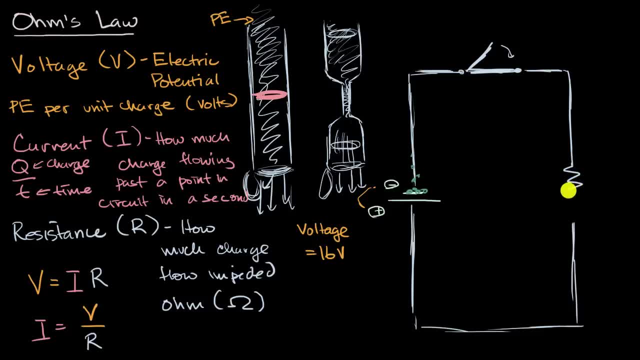 And so let me draw Resistance here. So that is how we denote it in a circuit diagram. And let's say the resistance here is eight ohms. So my question to you is: given the voltage and given the resistance, what will be the current through this circuit? 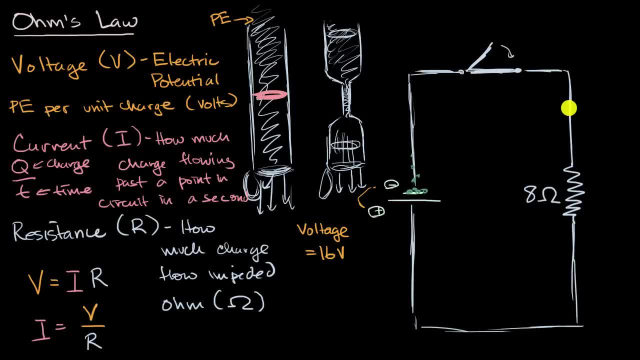 What is the rate at which charge will flow past a point in this circuit? Pause this video and try to figure it out. Well, to answer that question, you just have to go to Ohm's law. We wanna solve for current. We know the voltage, we know the resistance. 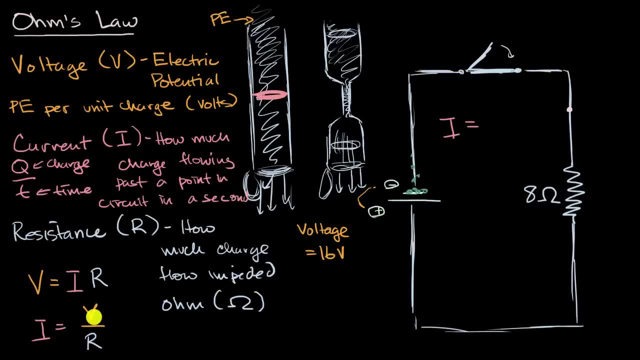 So the current in this example is going to be our voltage, which is 16 volts, divided by our resistance, which is eight ohms, And so this is going to be 16 divided by eight is equal to two, And the units for our current 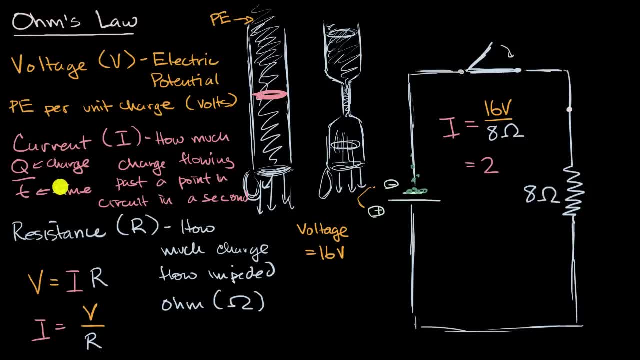 which is charge per unit time: coulombs per second. you could say two coulombs per second, or you could say amperes, and we can denote amperes with a capital A. We talked about these electrons flowing and you're gonna have two coulombs worth of electrons. 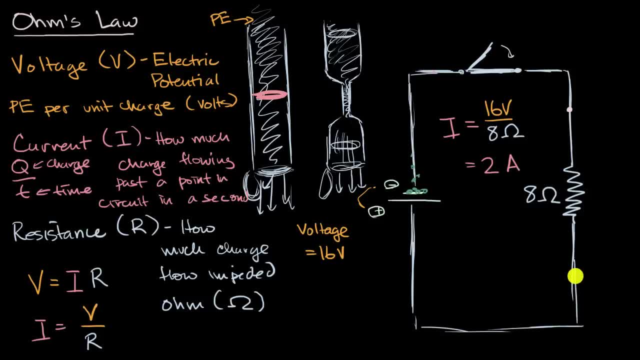 flowing per second past any point on this circuit And it's true at any point. same reason that we saw over here- Even though it's wider up here and it's narrower here because of this bottleneck, the same amount of water that flows through this part.